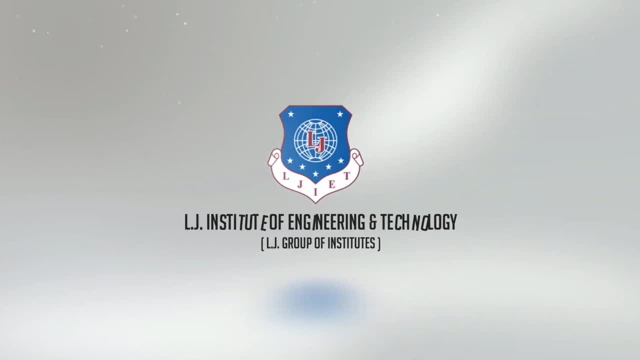 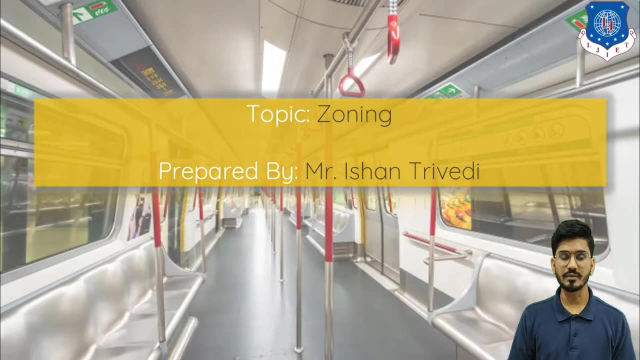 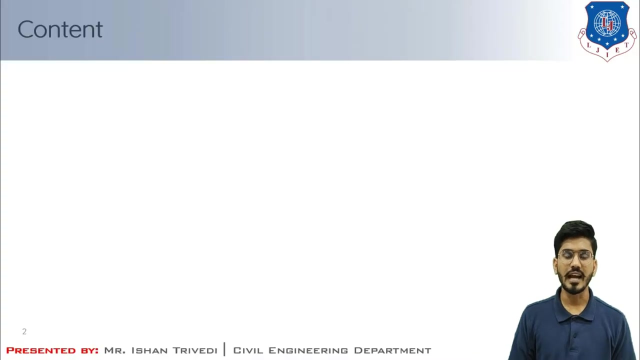 Hello students, I am Ishan Trivedi. Welcome you in the video lecture 6.. Today I am going to discuss about zoning. In this session I am going to cover introduction and definition of zoning and its importance. Then basic movement in the transportation survey, the network. 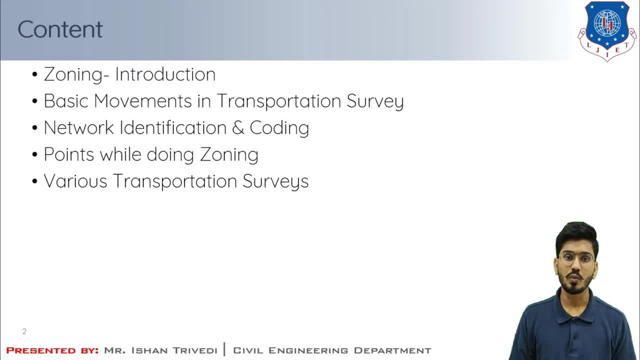 identification and coding, then points while doing the zoning and at last various transportation survey. So first we will understand what is zoning and its importance. The defined study areas is subdivided into smaller areas, which we call a zone, The term zone ordinarily referred. 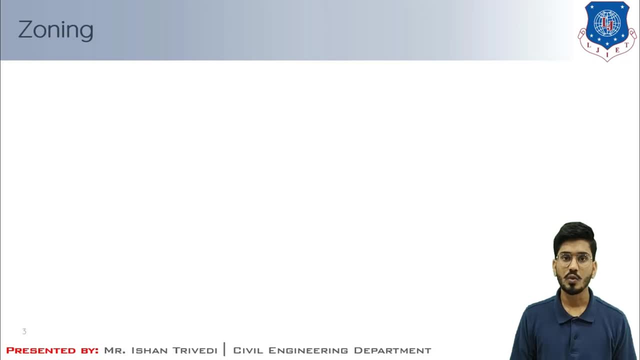 to a concentric ring or a belt with its central focal. Here the zoning is defined as the creation by law of sections or zones, such as residential, industrial, commercial, civic, institutional and recreational, in which the regulation prevents misuse of lands and buildings and limit their height and density. 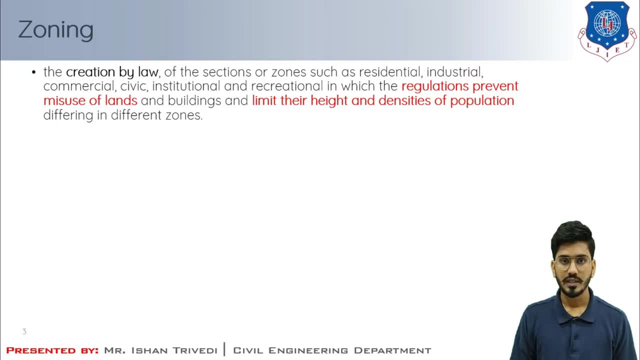 of population differing in different zones. Here what zoning does? zoning is the boundaries, which has been created by laws, and it covers the residential, industrial, commercial areas. and here the regulation has been done on imposing such a way that it prevents misuse of land and buildings, It limits the building heights. 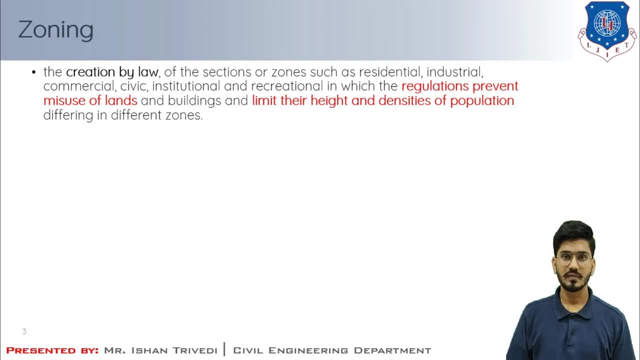 and the density of population. The definition is very simple. The definition of zoning is also, So now understand the importance of zoning, or you can say, advantages. Zoning sets apart the different areas in the town for specific purpose. It prevents the encroachment of one zone upon. 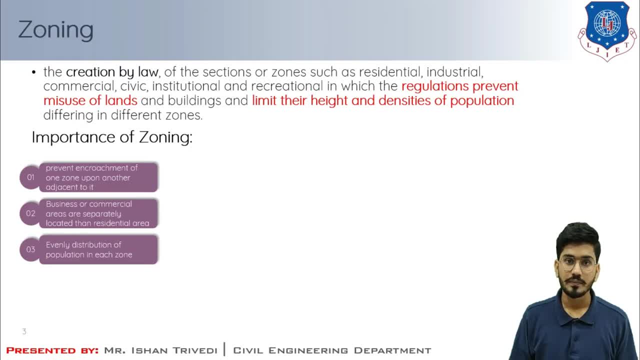 another zone or upon another adjacent zone. For instance, the industrial area is located away from the residential area so that it is not affected by the dangerous gases and smoke. Then business or commercial areas are also separately located, with their garages and service stations at distance from the residential area. As such, these residential 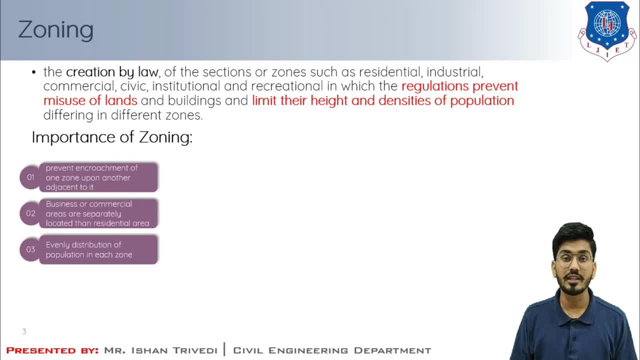 areas are free from noise and the road traffic. The population is distributed throughout the town By zoning regulations so that there is no concentration of population in any particular zone. That means the population is evenly distributed, and thus I will define the boundaries. Then, height zoning regulates the height of buildings and hence the high rise building. 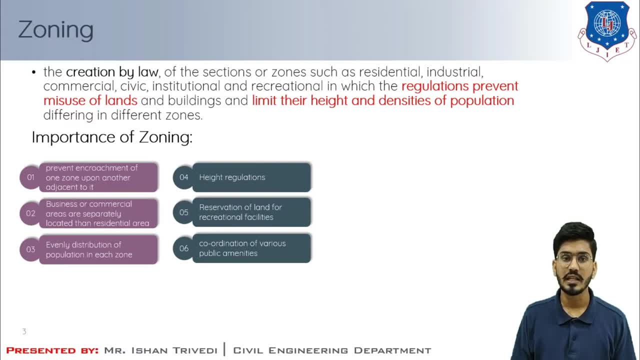 will not be allowed to construct near the small houses, Otherwise they will cut off the sunshine. air breeze Zoning helps in making the life of the resident uncomfortable. A land in the form of recreational area is also set aside for parks, playgrounds, stadiums. 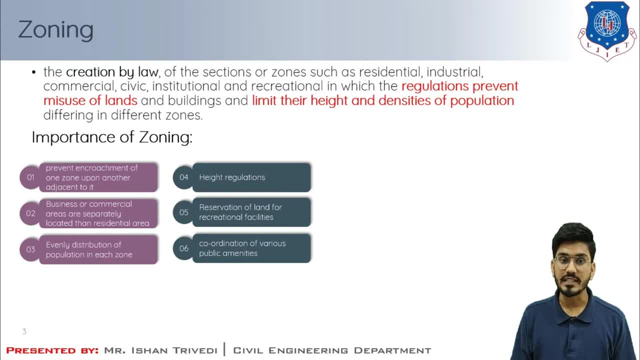 theatres and so on. In many of the cities, certain percentage of land has been reserved for these recreational activities. Now, zoning helps the proper coordination of various public amenities like water supply, drainage, electricity water supply and so on. Zoning helps the proper coordination of various 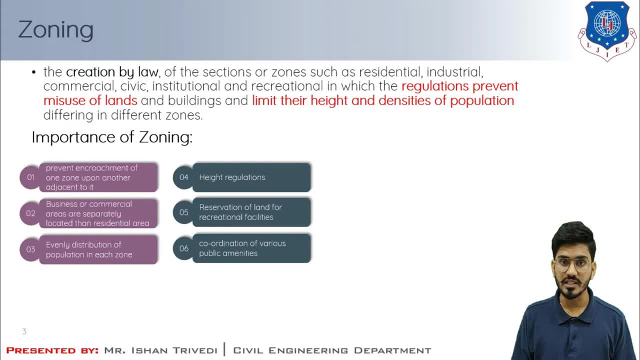 public amenities like water supply, drainage, electricity and so on. Zoning helps the proper coordination of various public amenities like water supply, drainage, electricity and so on. Zoning also ensures planning게요的. Zoning also helps the properaminate functioning of large 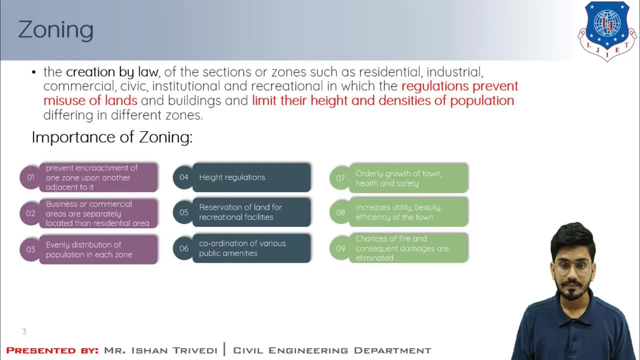 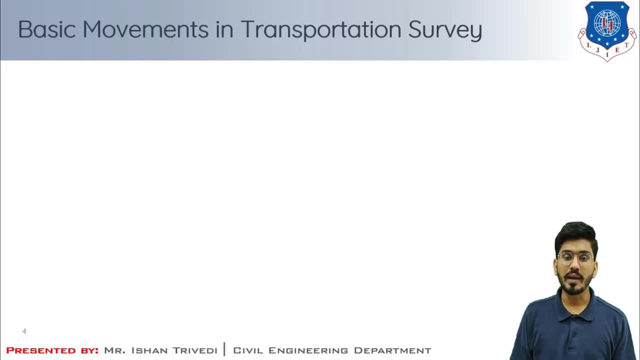 Usages such as buildings, renewable, are also eliminated. so these are the advantages of zoning. now understand the basic movements in this transportation survey based on zone. the purpose of zoning is to facilitate the spatial quantification of land use and the economic factors which influence the travel pattern. the data collected on the 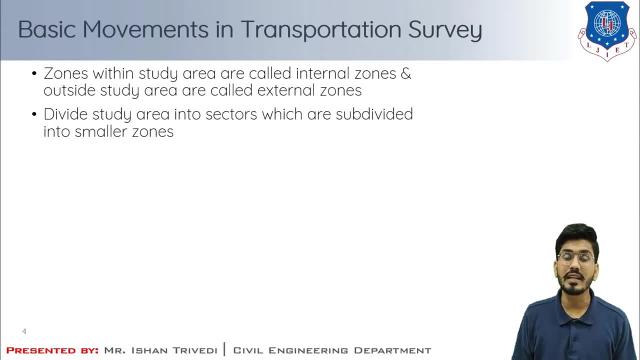 individual household basis cannot be conveniently considered and analyzed unless they are aggregated into smaller zones which reflect the average characteristics of individual household zoning also helps in the geographically associating the origins and destination of travel. zones within the study area are called internal zones and those outside the central. 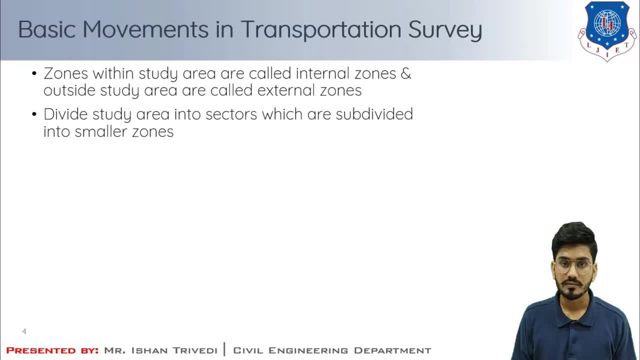 area are called internal zones and those outside the central area are called the study area, are called external zones. or you can say a cordon line is there or a boundary is there and outside that area is called external zone. in the large study project it is more convenient to divide the study areas into sectors and 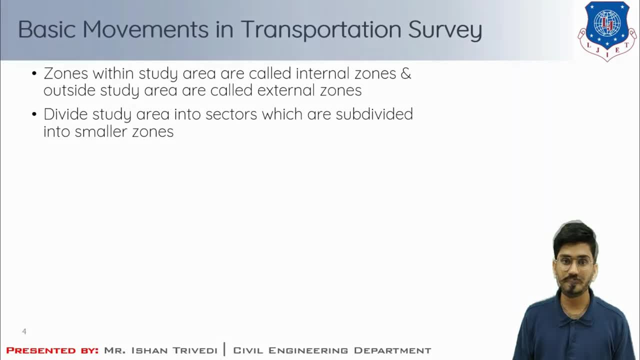 which is further subdivided into smaller zones. in addition to the external cordon lines, there may be number of cordon lines arranged as a concentric ring to check the accuracy of the survey data, and the screen lines which are running through the study area are also established to check the 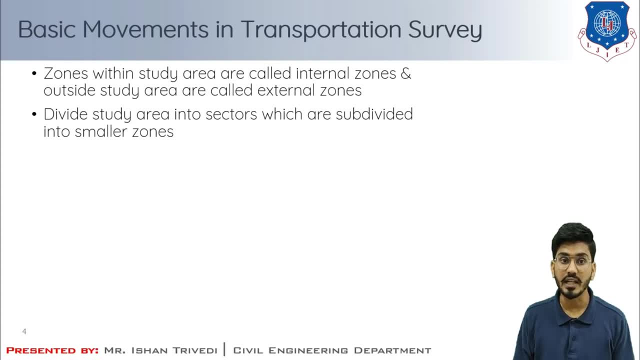 accuracy of data which we have collected from the home interview survey. again, I am repeating the screen line. I am quoting this: the screen line running through the study area is established to check the accuracy of data that we have collected on the survey. data screen lines can be conveniently located along the physical or a natural barrier, having few 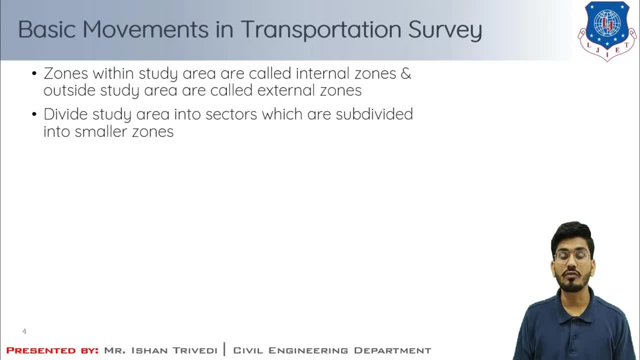 crossing points, for example the barriers of river canal, railway line or any hug. so, as I told you, three to four term, that is, of internal zone, external zone, screen line, cordon line. now I these are the geographical feature or phenomenon which restrict or which identify the survey area and based on that, or based on the basic moment, the types of survey are of internal to internal surveys, then internal to external survey, external to internal survey and, at last, external to external survey. for a large urban area, the internal to internal survey in involves more movements, whereas for small areas having population less than 4,000, the internal to internal travel is less. 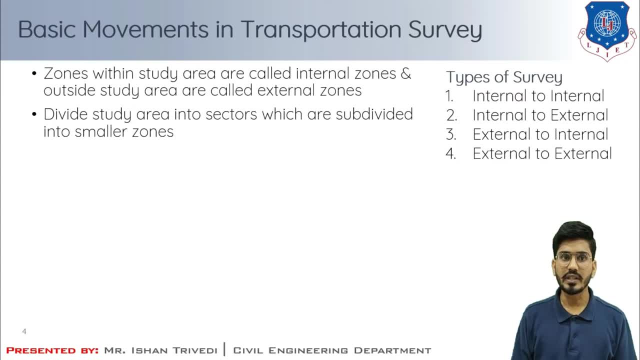 significant. the internal to internal travel is based, studied it by the home interview technique which checks by the screen line survey. here you can see a screen line which is the outer peripheral line of any study area which is further divided into the cordon line which are blue highlighted cordon line and each cordon line is further divided. 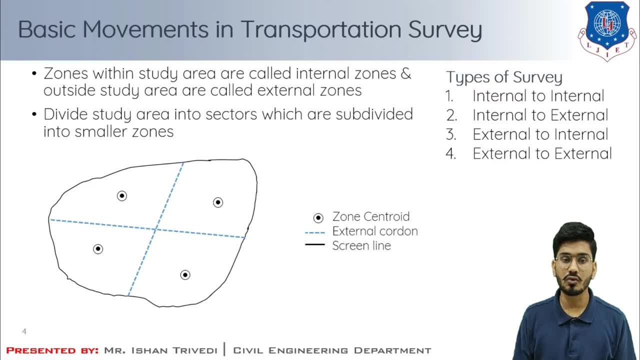 into zones. so here, four zones are there and their centroids are there. now, here, as I said, there is an internal to internal movement. for larger area, these are of heavy, or you can say more in numbers, and for lesser, in the smaller area. this trial, Peter, is based, studied it by the home interview. 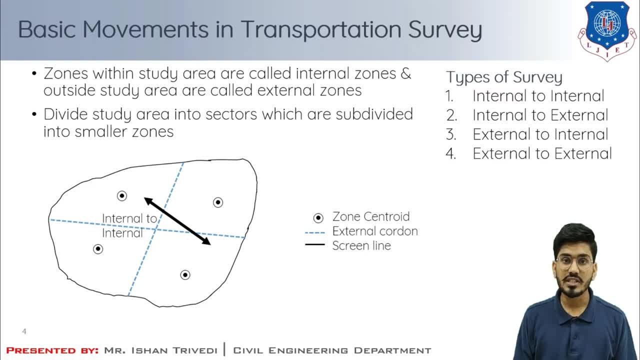 technique and will get those checks by the screen line. so similarly we can do the internal to external survey, external to internal survey and external to external travel, which is studied by the cordon line server. the surveys can take, collect many data which are in the form of at home, during the trips and at the destination. 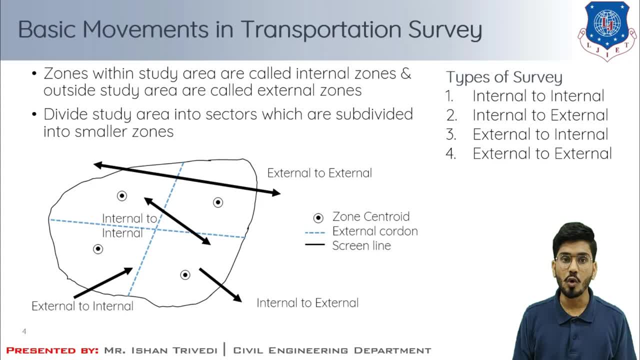 end of the trips. The data collected at home can be wide ranging and can cover all the trips which are made during a given period of time. The data collected during the trip is necessarily of limited scope, since the procedure yields data only on the particular trip that are of intercepted means, here the during trip. 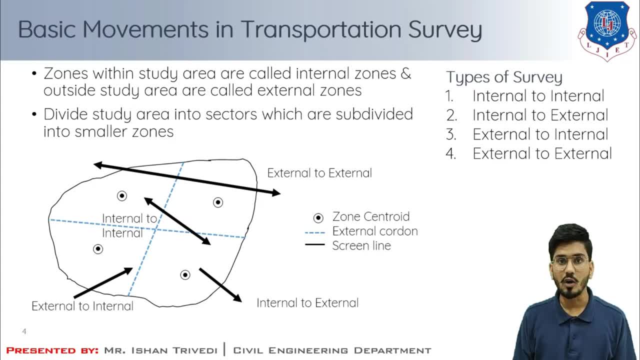 data collection is of limited in scope and I will get the data of that particular trip only and at destination end, the data collected by the direct interview, provided by the data on demand for, such as parking facilities, and on major traffic attractors, such as offices, factories. 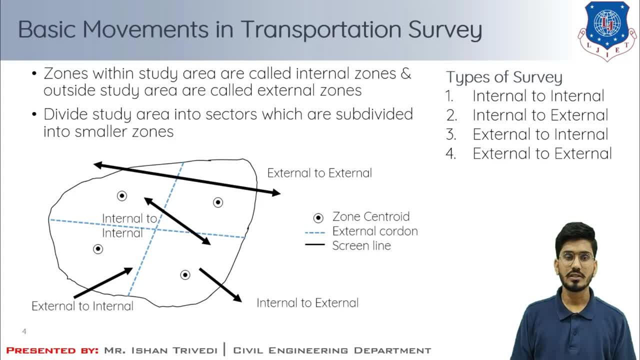 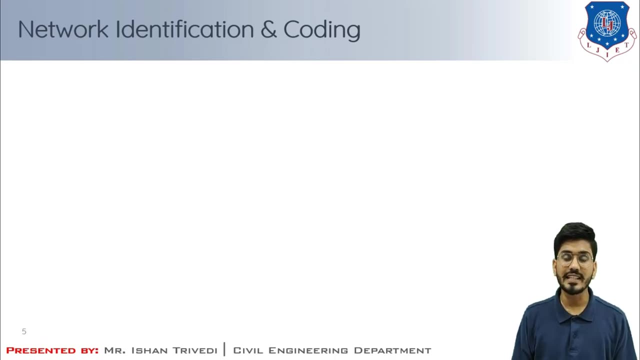 commercial establishment and so on. So this is the types of survey and the basic moment of transportation survey. Now understand the network identification and its coding. For coding and for easy data availability or to manage the data easily, we have to identify the spots or the study area. 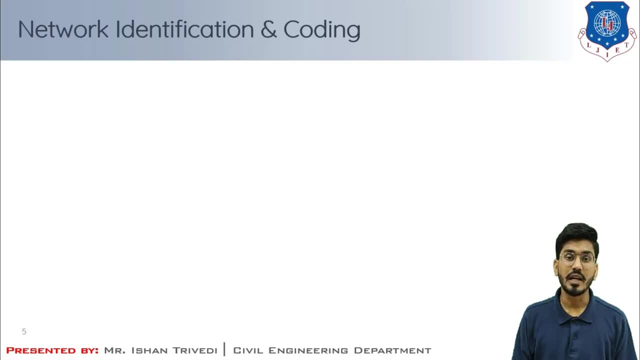 So that their interpretation of the data can be easily managed. And for that zones, their sectors and sub zones, has been given particular class of coding. For coding of zone, a convenient system is applied and it will be very useful for the study, For example, in a study area. one such system is to be divide the study area into various 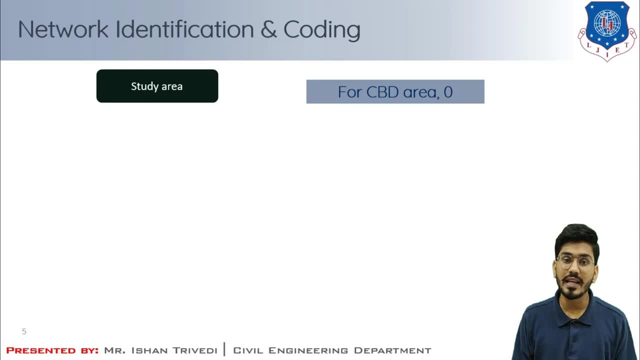 sectors For central or you can say for civil area. For central or you can say for civil area, For CBD area it is designated as zero and remaining eight are designated to the study area. or you can say those sectors in clockwise manner: Here total 0 to 8 number are there in that zero is denoted to CBD area and rest 1 to 8. 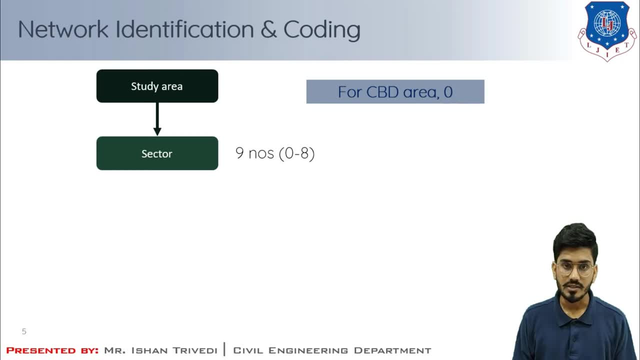 are designated to the sectors And for a particular sector. this is a different substitution and for a particular zone category, we can say: for CPD area, it is designated as 0 and remaining 8 are designated to the study area. For CPD area, it is designated as 0.. 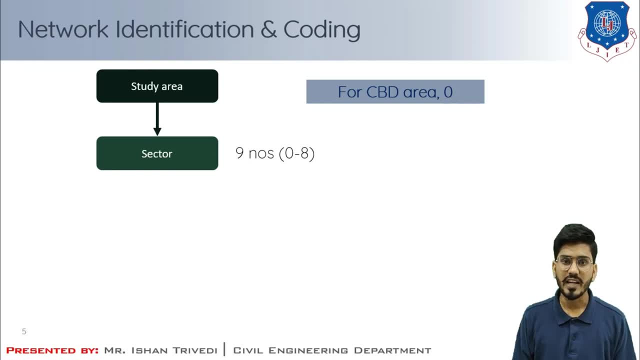 For example- here I am giving a 5 number for the sector- Then in that prefix, 9 is reserved for external zone. Now, furthermore, each sector is subdivided into 10 zones bearing the numbers of 0 to 9. you can see here: 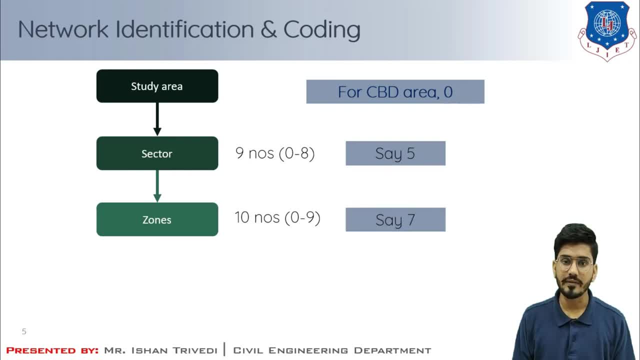 For this zone, I will provide a number, say 7.. Then, similarly, these zones are furthermore subdivided into subzone, which denotes the digit ranging from 0 to 9 having 10 numbers. Say for this is a 2. Then a subzone comprises with 3 numbers, or you can say 3 digits. 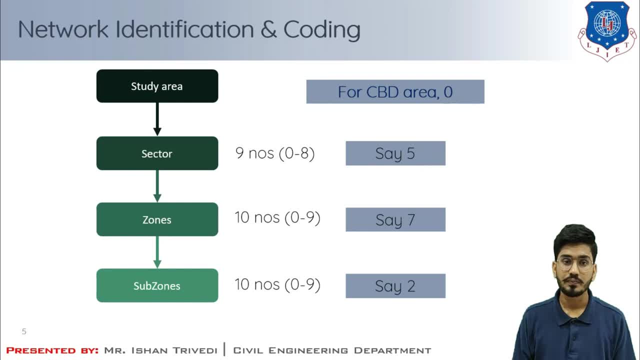 For example, here I have shown you, 572 means a subzone Bearing the number. 572 belongs to the sector 5, to zone 7, and in that zone there is a subzone of 2 number. And this is how you can do the coding for the network identification. 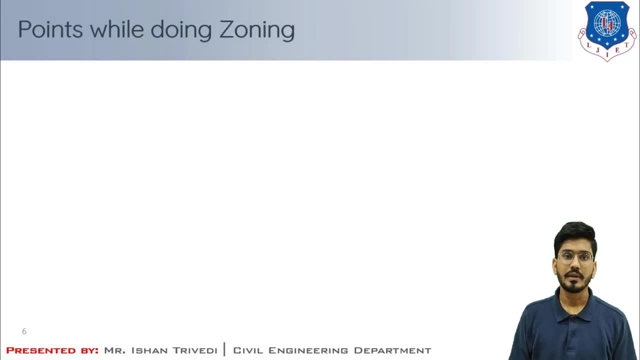 Now, at last, points to be kept while doing the zoning Here. first is the land use is the most important factor in establishing the zones for transportation survey, And the predominant land use for establishing those zones are of residential, industrial, commercial, recreational and open space. 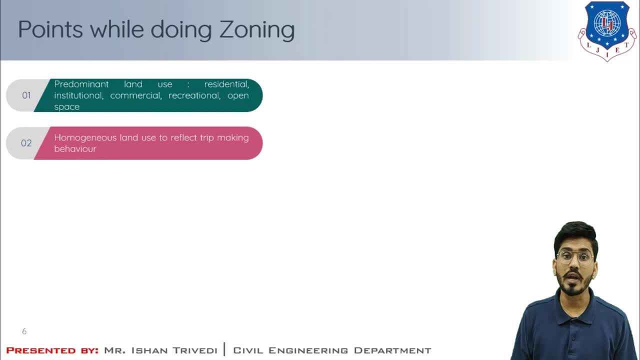 The zone should have a homogeneous land use so as to reflect the accurate the associated trip making behavior. While subdividing the study area into zones, the anticipated changes in the land use should be considered. The zone should not be too large to cause the considerable error in the data. 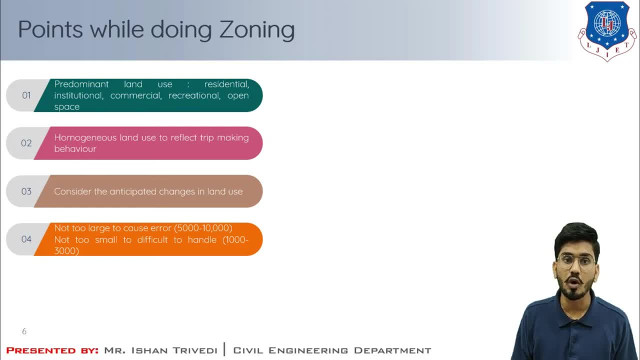 and at the same time they should not be too small to cause difficulties in handling or analyzing those data. As general rule, a population ranging from 1000 to 3000 may be optimum for the small area and maximum population 5000 to 10,000. 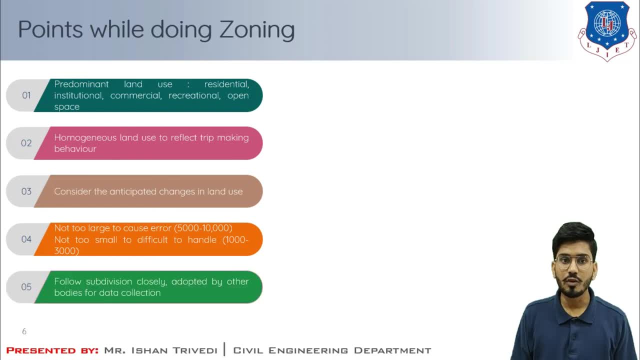 for the large area It would be advantageous to follow the subdivision closely that adopted by the other bodies for data collection. For example, for census of India, the data collection is being done in the Ahmedabad, in the particular ward. Similarly, those ward or those area will be followed by the municipality or local governance. 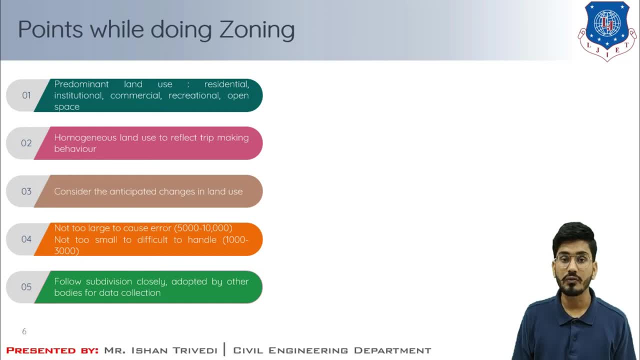 And this will facilitate the correlation of data. The zone should not be too large or too small. The zone should not be too large or too small. The zone should be, or should preferably have, regular geometric form for easy determination of zonal centroid, which represent the origin and termination of travel.